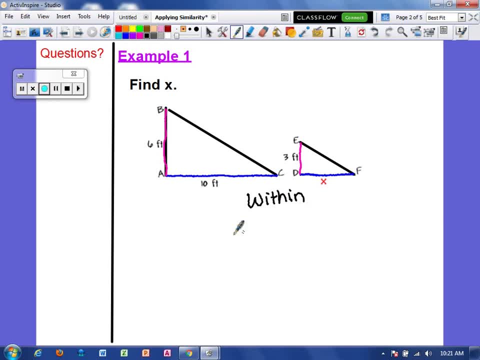 particular problem. I'm going to set up a within ratio, So I'm going to go within the same figure and I want to make sure x is included. So I'm going to start with this. So let's say I'm going to put pink over blue. All right, pink over blue, that would be three over x. And I'm going to go. 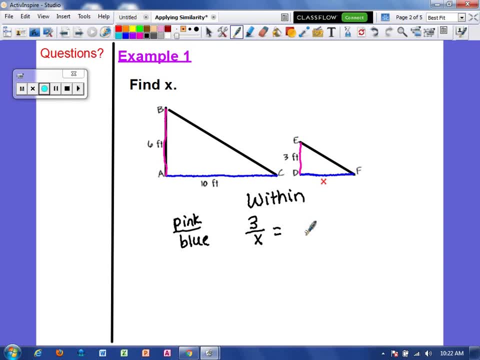 to the large triangle. and I'm going to do the same thing. Pink over blue, six over ten, And now we will cross, multiply and solve. So three times ten equals 30. And six times x equals 6x. I'm going to 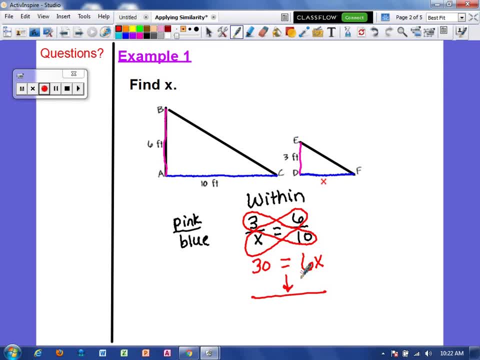 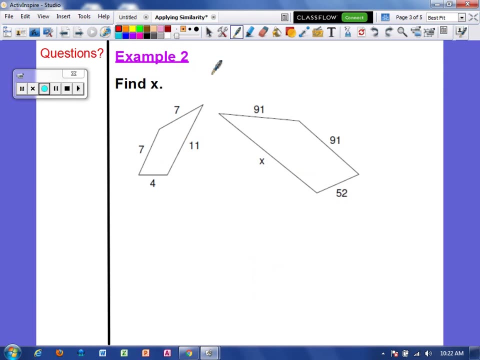 set those equal to each other And then divide by six. on each side, 30 divided by six is five, So this side equals five feet. All right, again Example 2, I'm going to go ahead and find the missing side. 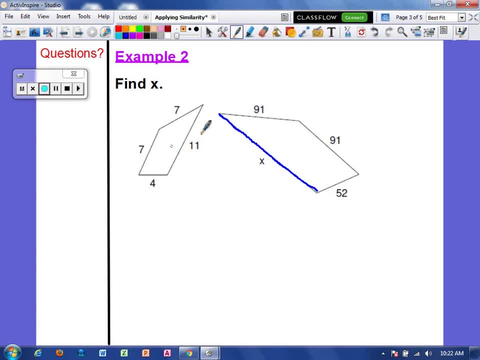 Now the corresponding side on this figure would actually be the right side, because it has been flipped around, so be careful with that. Alright, so I found these corresponding sides. Now I just need one more pair so that I can set up a proportion. 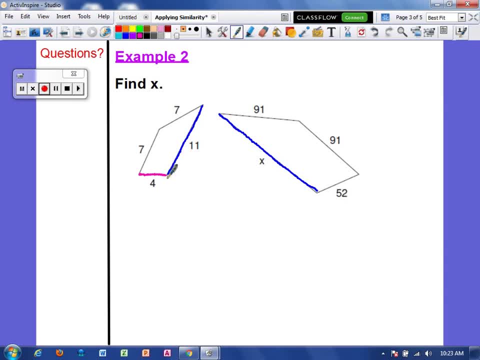 I am going to go with the smaller sides, So 4 will correspond with the 52 on the other figure. Now, on this particular example, I'm going to set up a between ratio, So I'm going to go from one figure to the next. 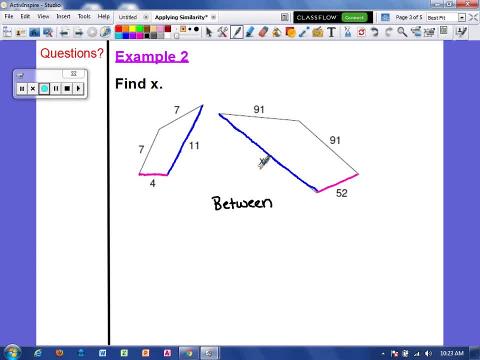 So, since I want X involved, I'm going to start with X. So I am going to go from the big to the small figure. Alright, so I'm going to put in the middle. I'm going to put X over 11, because that's its corresponding side. 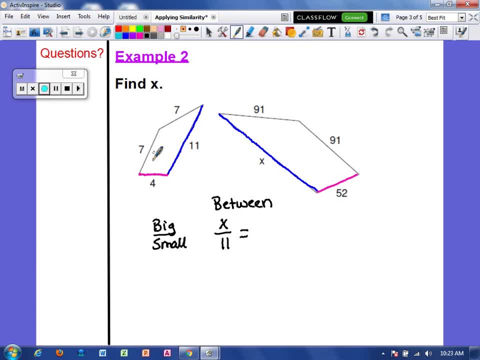 And then I'm going to go back to the big figure and put 52 over its corresponding side of 4.. 52 over 4.. Now we're going to cross, multiply and solve. 4 times X equals 11 times 52.. 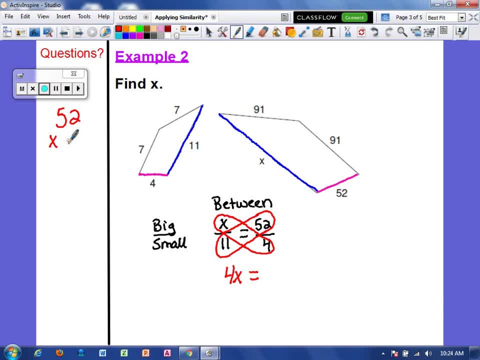 Let's come over here and work that out: 2 times 1 is 2.. 5 times 1 is 5.. Put the placeholder: 2 times 1 is 2 and 5 times 1 is 5.. And then we're going to add that together. 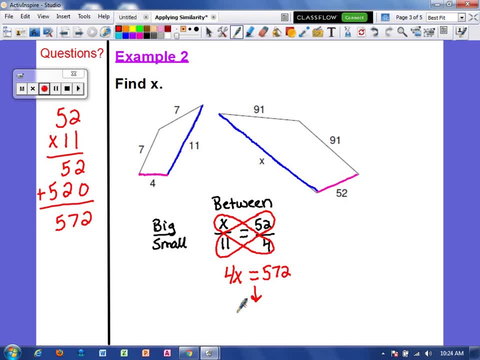 So 4X equals 572.. We're going to divide by 4 on each side And again let's come over here to the side and work that out: 4 goes into 5 one time, 4 goes into 17 four times and 4 goes into 12 three times. 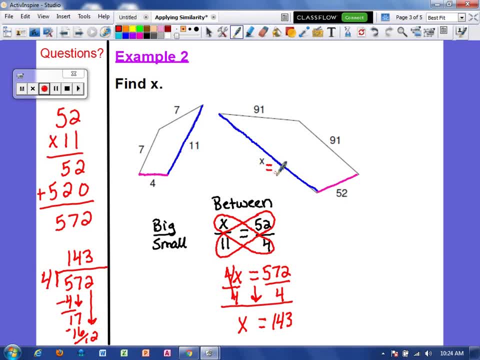 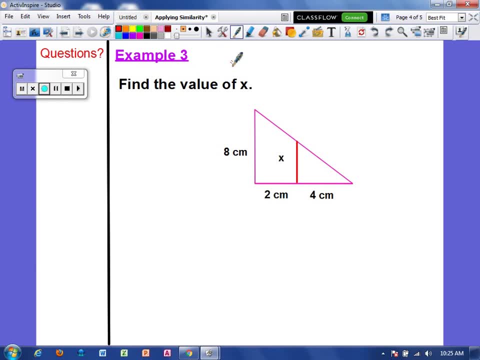 So our missing side would measure 143 units. Alright, example 3. Find the value of X. So we've got one triangle inside the other. So we're going to find the value of X. So we've got one triangle inside the other. 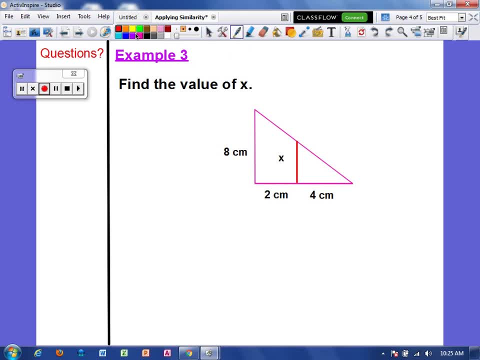 So let's go ahead and identify where our missing side is. So this is our missing side And that's already shaded red, So I am going to find its corresponding side. So on the big triangle, the corresponding side would be the side that measures 8 centimeters. 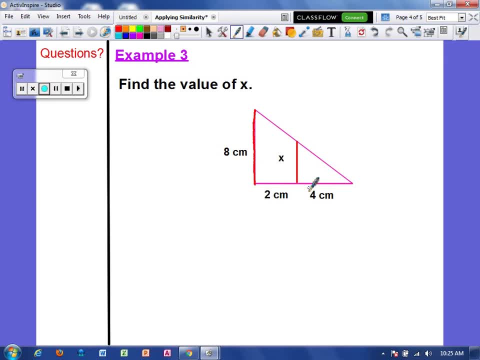 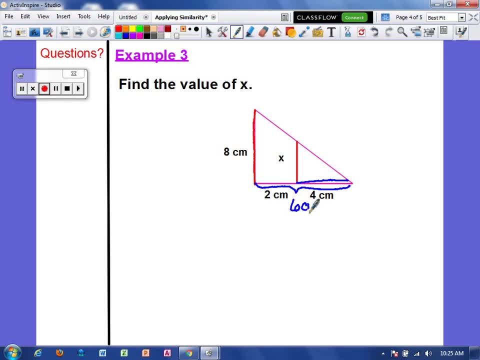 So this is going to correspond with this whole side on the larger triangle, which is going to measure altogether 6 centimeters, 6 centimeters. On this particular problem, I'm going to go ahead and set up a within ratio. So I am going to go, I'm going to put the red side over the blue.